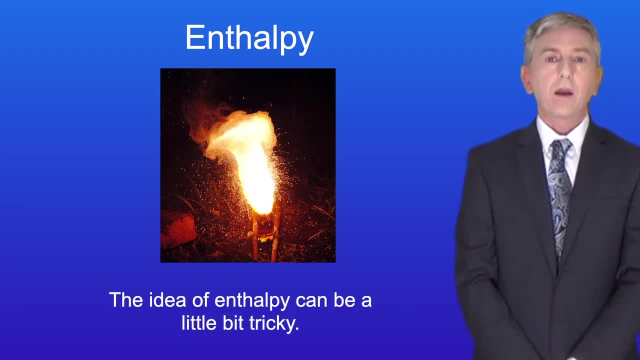 symbol, capital H. Now the idea of enthalpy can be a little bit tricky. Enthalpy refers to all the heat energy that's stored in a chemical system, And the words chemical system mean all of the chemicals present in the reaction. Now the problem is that enthalpy is very difficult to determine. So instead, scientists 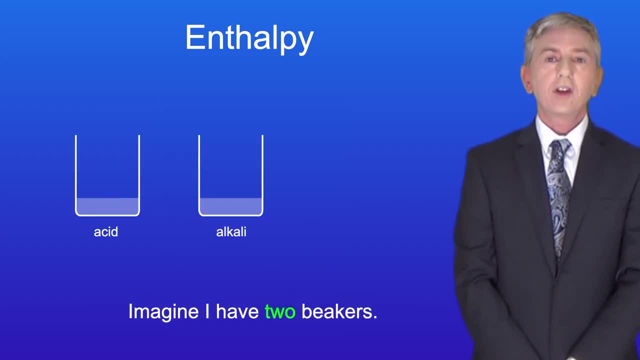 determine the change in enthalpy. Imagine: I've got two beakers. One beaker contains an acid dissolved in water and the other beaker contains an alkali dissolved in water. If we mix these two beakers together, then neutralization takes place. Now neutralization reactions release heat energy. So if we measure the 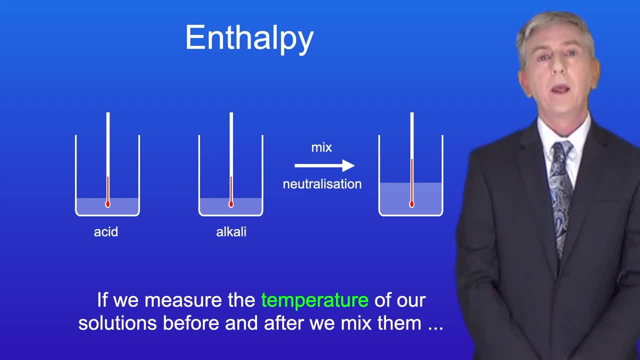 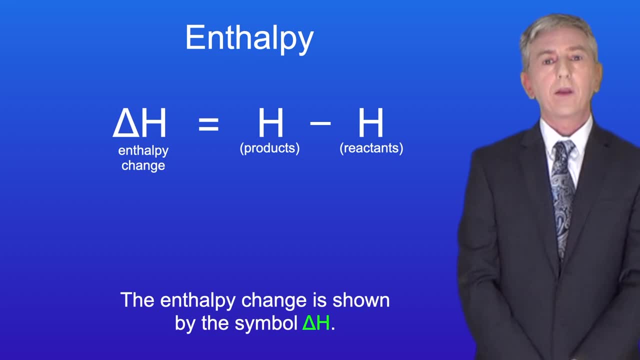 temperature of our solutions before and after we mix them. then the change in temperature can be used to calculate the enthalpy change. The enthalpy change is shown by the symbol delta H. The triangle is the Greek letter capital, delta, and this means change in. So delta H means change in enthalpy, And this 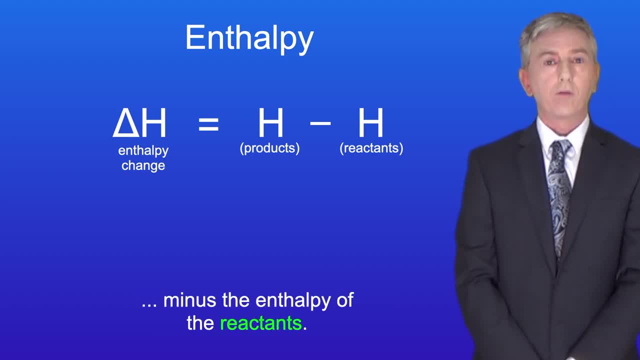 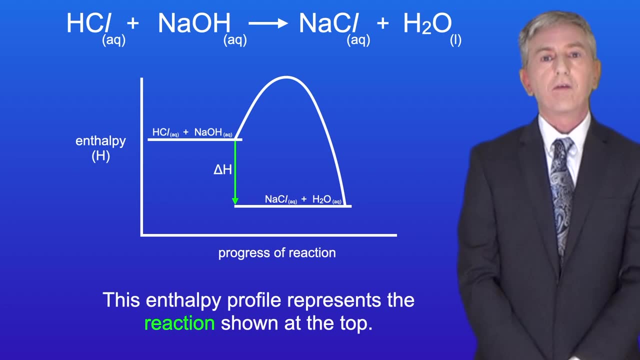 represents the enthalpy of the products minus the enthalpy of the reactants. Now we can represent enthalpy changes on a profile like this. This enthalpy profile represents the reaction shown at the top. This is the neutralization reaction between an acid and an alkali that I discussed earlier. 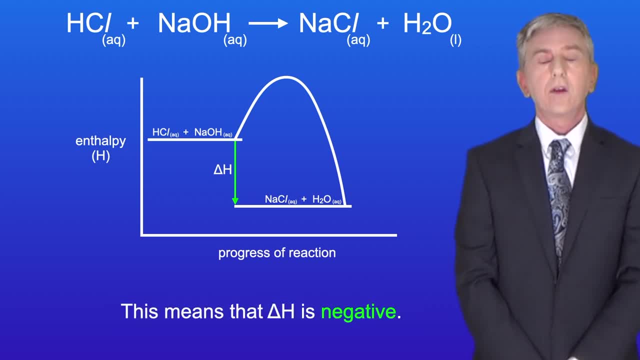 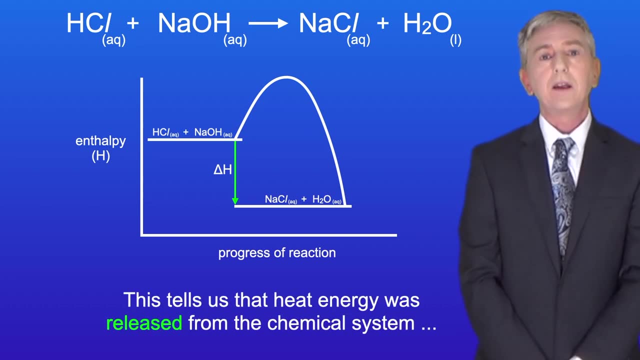 As you can see, the enthalpy of the product is less than the reactants. This means that delta H is negative And we show this with a downward pointing arrow. This tells us that heat energy was released from the chemical system to the surroundings. 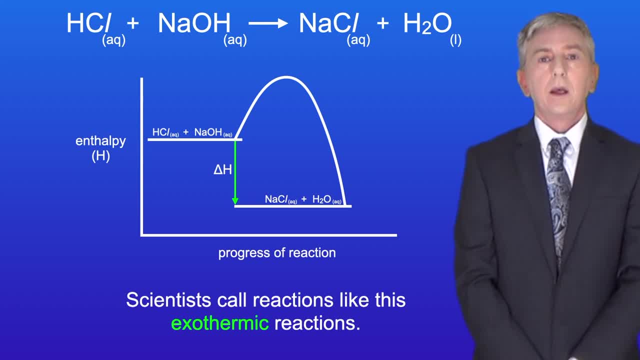 Scientists call reactions like this exothermic reactions. Now, in the case of this reaction, the chemicals are dissolved in water, So the surroundings are the water that the reaction takes place in, Because heat energy has passed from the chemical system to the surroundings- the temperature. 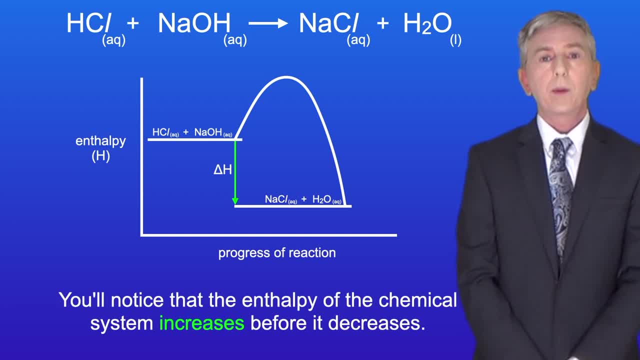 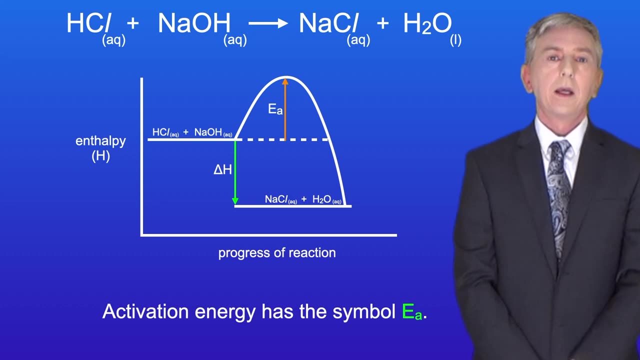 of the surroundings will increase. You will notice that the enthalpy of the chemical system increases before it decreases. This increase is called the activation energy and we show that on the diagram. like this, Activation energy has the symbol capital, E, lowercase, a. Now, in order for any reaction to take place, we start by breaking the chemical bonds in